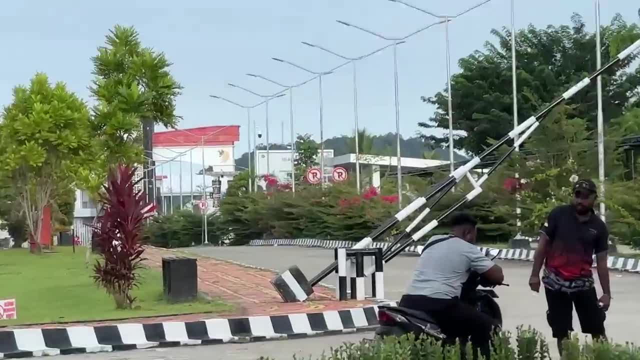 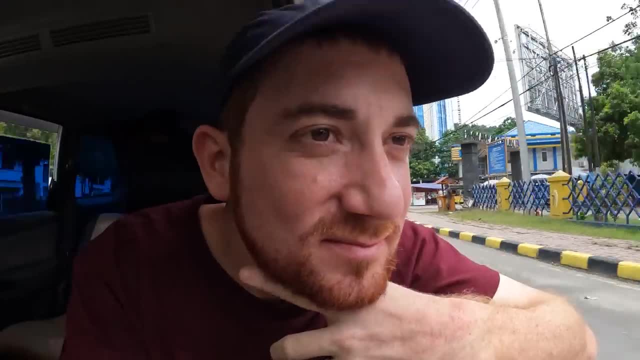 I have to get out of the Indonesian side of Papua Island right now and cross the border into the other side, which is Papua New Guinea. I have a lot of incredible stories planned in Papua New Guinea and I'm really excited to get there. 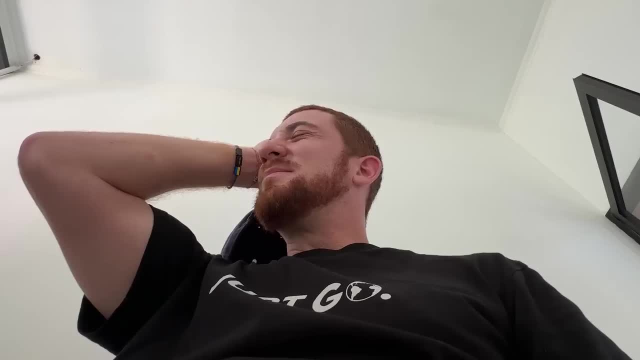 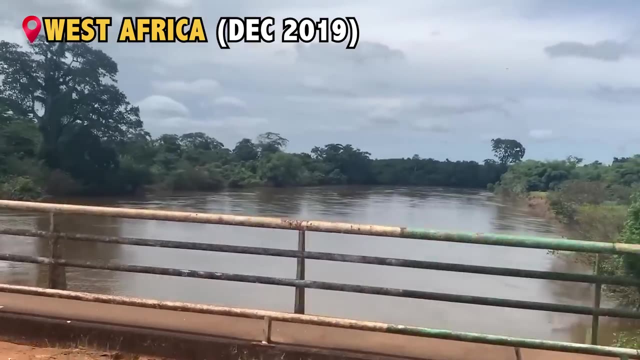 But I must cross the land border, which will not be easy. In many ways, Papua Island reminds me of my road trip across West Africa in 2019.. Welcome to Sierra Leone. There's lots of bribery, corruption and overall chaos on the streets. 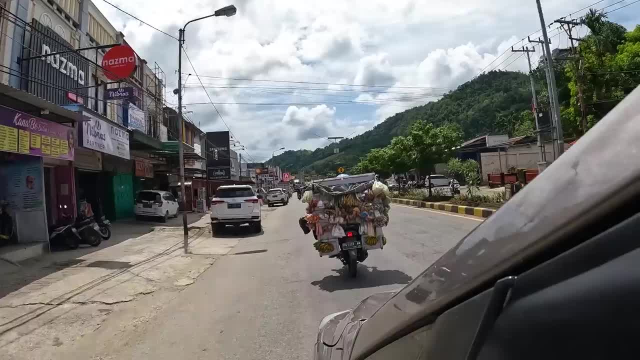 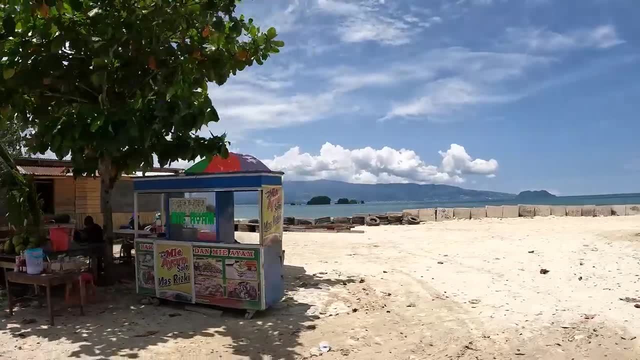 So what I'm trying to say is that this is going to be one hell of an adventure, And it starts with a two-hour drive to the physical land border. Look at the beautiful nature, man. This beach is amazing. Look at that. 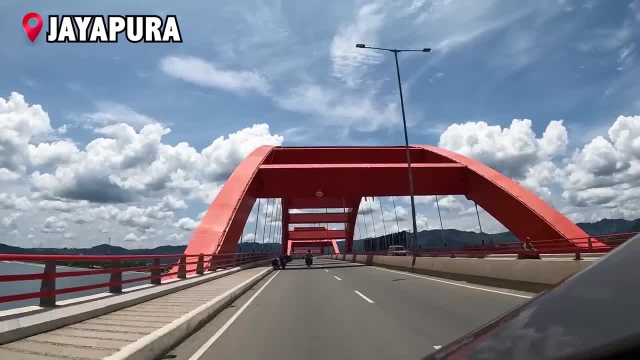 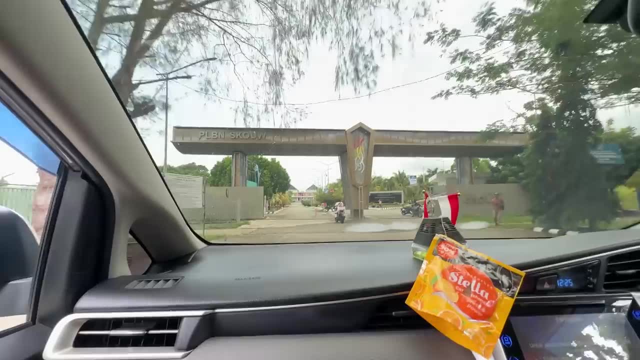 We're going over this amazing red bridge. This is the iconic symbol. This is the iconic symbol of Darapora: the bridge. I think we're close to the border. Yeah, We've officially arrived to the border town. I haven't crossed the land border in many years. 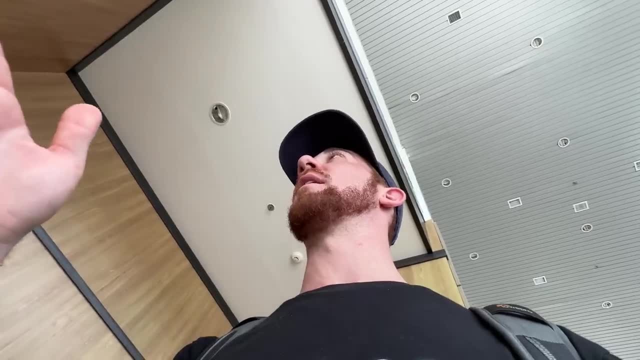 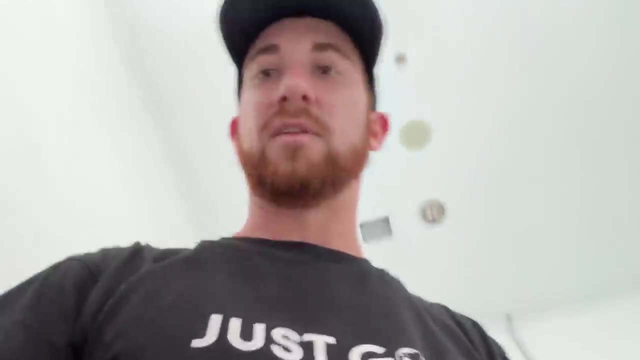 So how can I enter PNG? I really need to enter PNG today. Can we call someone or can you go investigate? This is crazy. I've never heard this happening. They just told me that if they stamp me out of Indonesia, then I can't get into PNG. 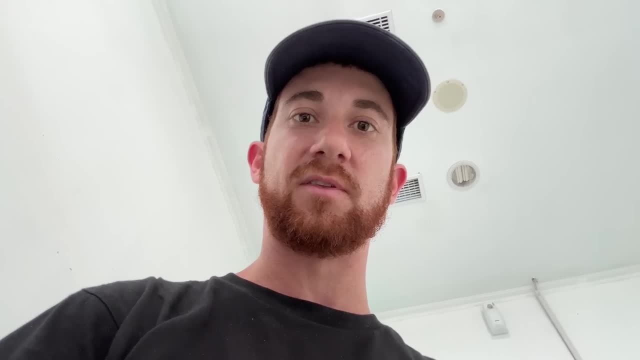 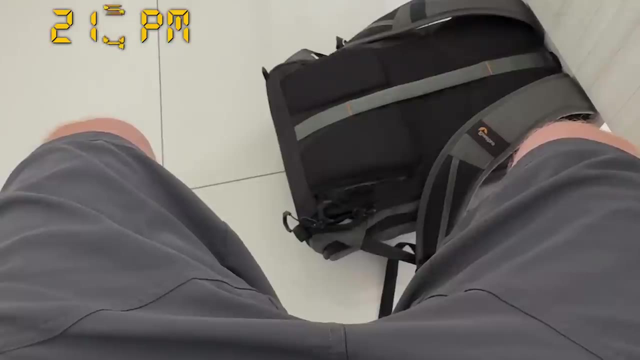 because there's nobody working at the border control. There's no police officers there. They said they were out drinking late last night. I can't make it up. Maybe I don't need to stamp for PNG, I can just go. Then you will get arrested. 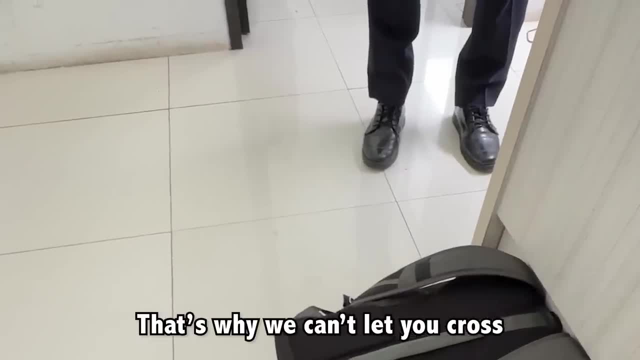 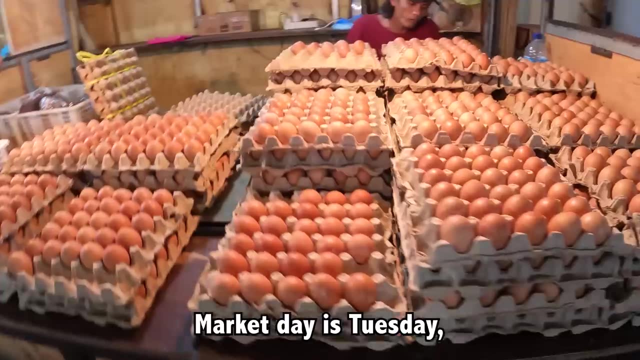 I will get arrested. Yeah, That's why we can help you cross. I know, Is this normal, Usually during 5 days. 5 days, By the way: it's Tuesday, Thursday and Sunday, So 3 days a week. 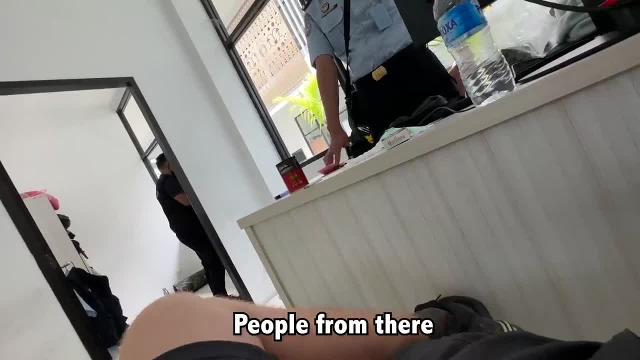 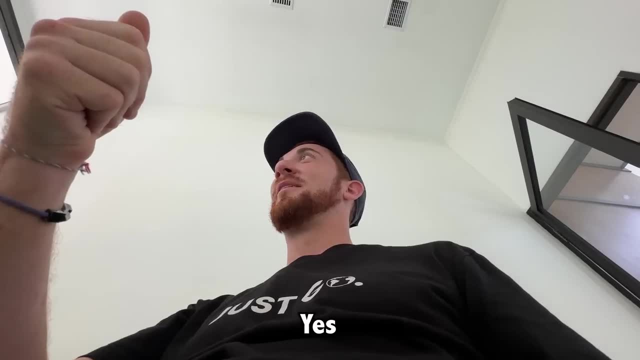 Yes, They drink too much and they don't show up to work People from there. they like to shop and sell. Yes, But some people like me need to cross the border. Yes, When I look out the window, I can see PNG. 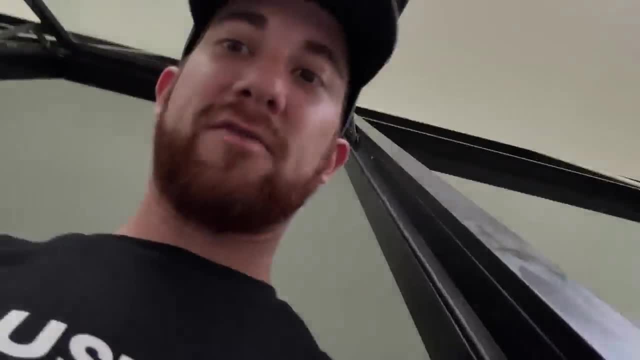 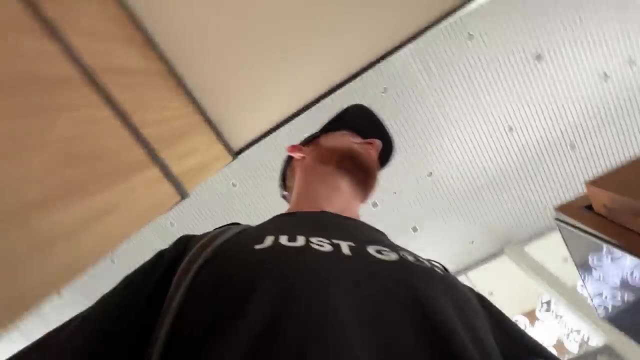 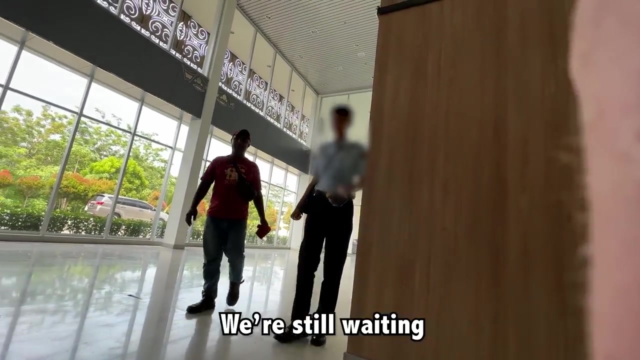 Right there, Right there, Over that fence, The border closes in 30 minutes and still nobody's here. Hey bro, What happened? What did they say? There's no police there. There's no officer there. Yeah, We are still waiting. 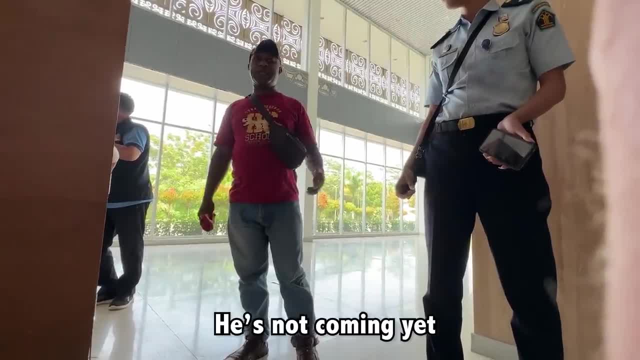 Maybe there's an officer with a stamp: Yeah, Is he coming? He's not coming yet, But he is coming. That's why they're going to wait. They're going to wait for you, But he will come. It's not confirmed. 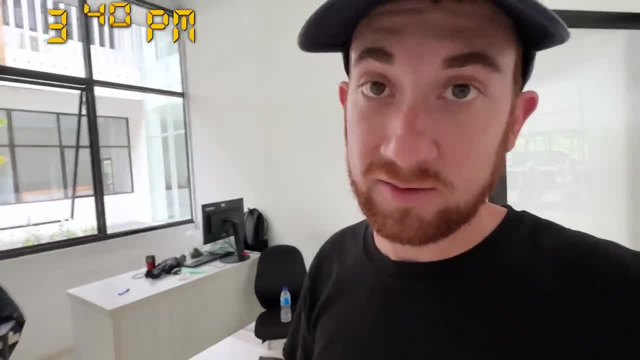 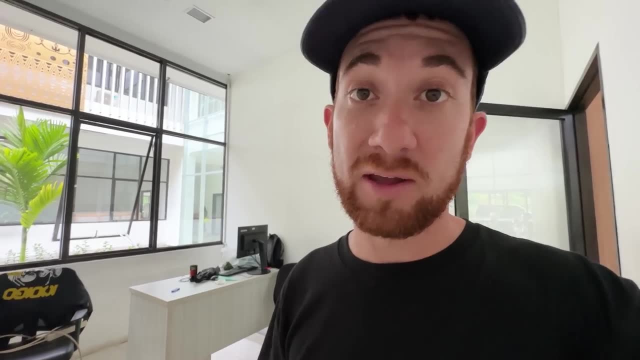 It's not confirmed. Well, it happens, And sometimes it doesn't always go your way. If I don't find out in the next 20 minutes, the border is closing And if no one's there in the PNG said to get me, I'm going back to Jaipur. 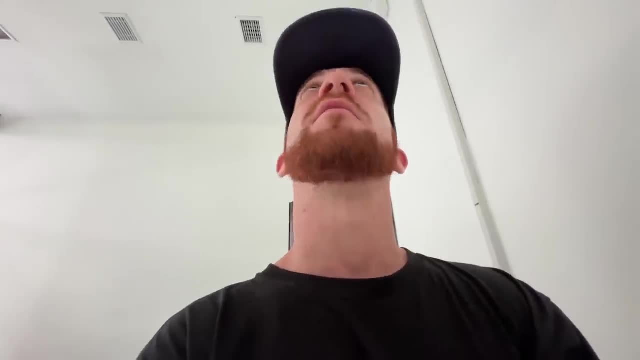 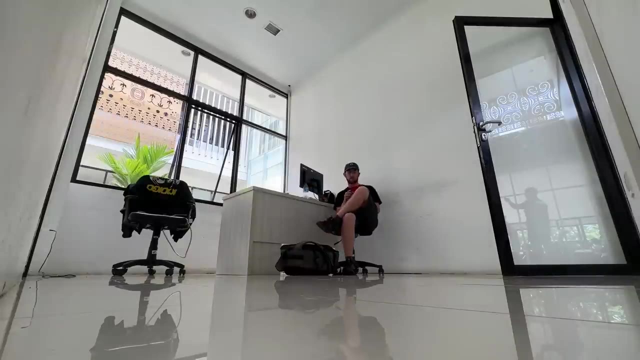 And then I'll probably just fly out tomorrow to Japan, Because it's too risky to go to PNG Tomorrow. the same situation might happen And I can't risk it. Please help me, bro. I need to cross today. If I don't cross today, it's a big problem. 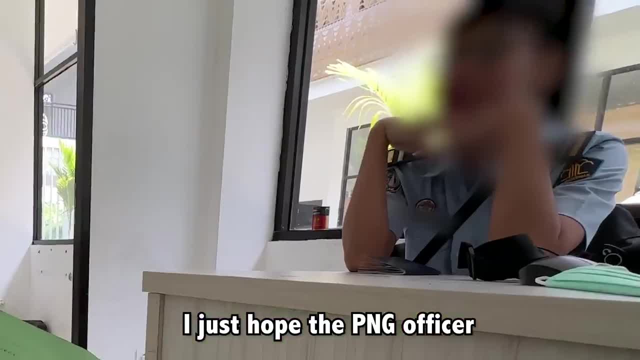 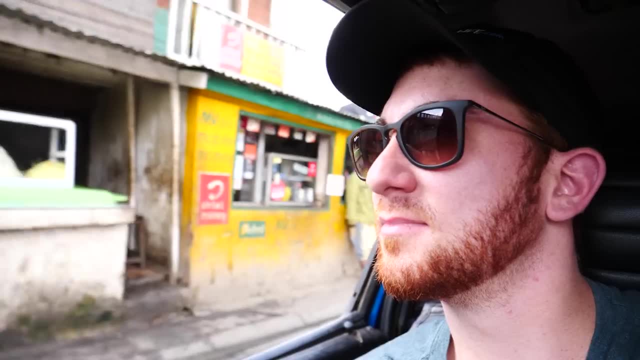 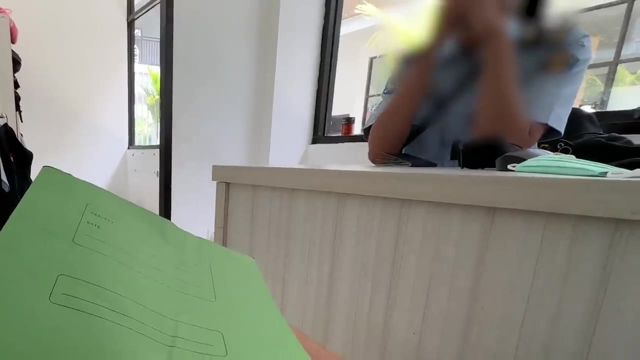 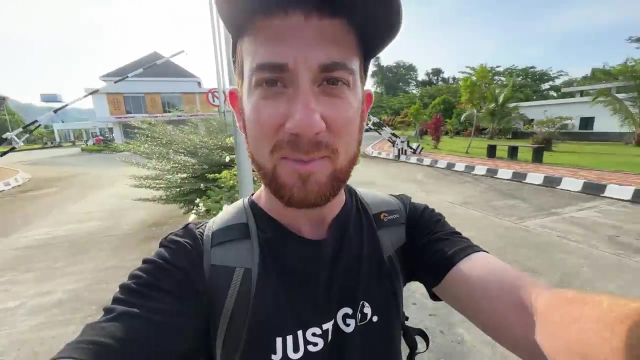 Because I need to fly. and it's Yeah, man, It's crazy, right. I travel many countries. I never had a problem where the immigration officer is not there to stamp the passport: He's drinking it. I'm stuck in no man's land between Indonesia and Papua New Guinea. 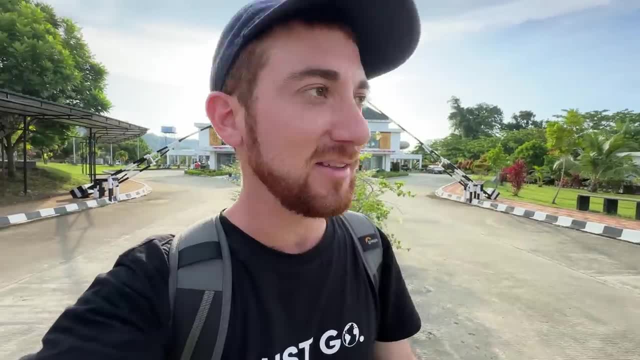 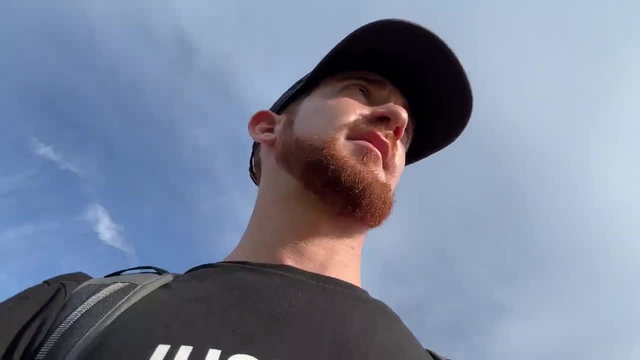 This is so annoying. If I can't enter Papua New Guinea in the next five minutes, I'm going to have to cancel my whole trip. All right, Hey, close the gate. Yeah, Nice to meet you. See you next time. 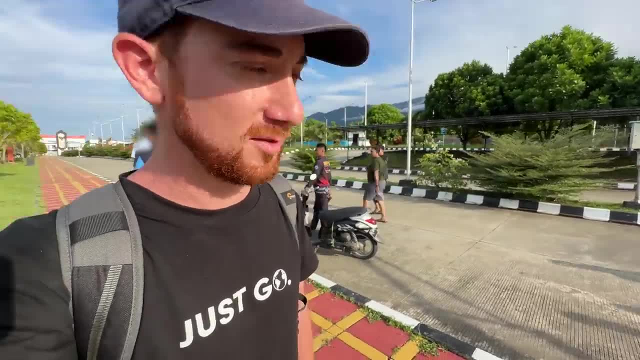 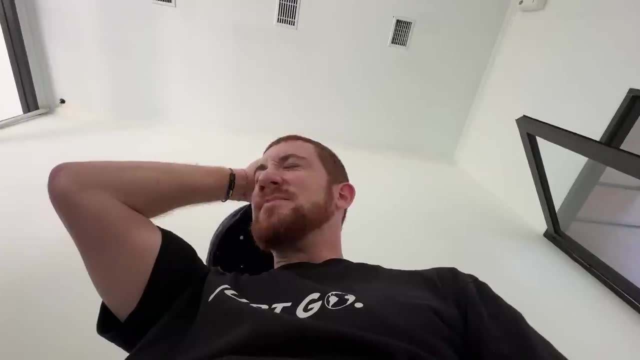 Meanwhile, all these people are crossing The market, people, the locals, But I'm stuck. I just got the word that the border closed on the PNG side and we're done, We're out. Well, you win some and you lose some. 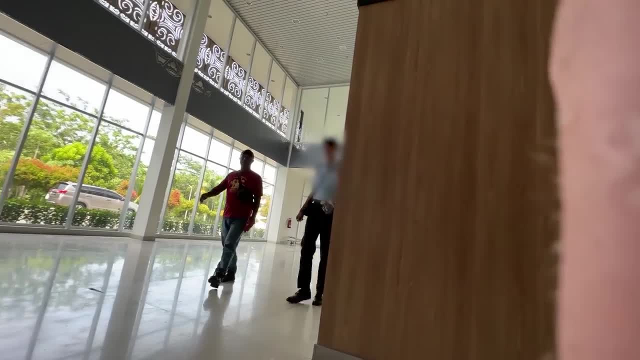 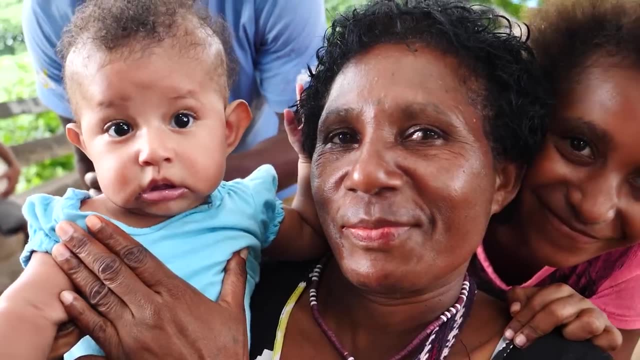 And I certainly lost this battle. It doesn't happen often, But when it does, it really sucks. There's nothing more that I want right now than to go into Papua New Guinea and document the amazing tribes and meet the people out there, But unfortunately, because of their annoying immigration officers who didn't show up to work- 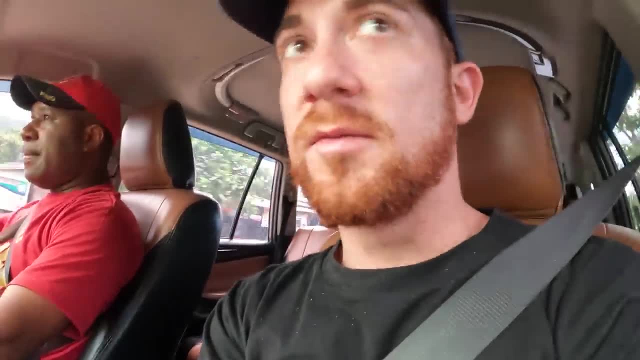 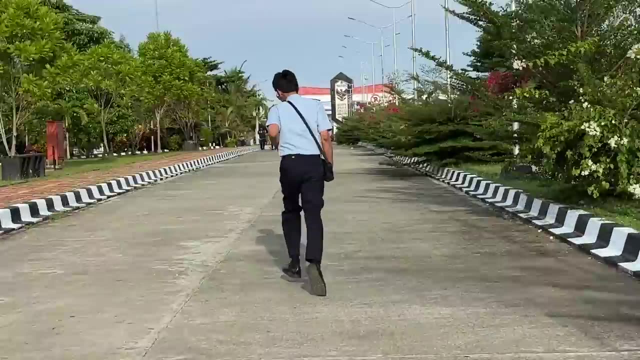 I got shafted. If you are a traveler and you are planning to cross this land border anytime soon, beware of the same situation happening to you. I hope that this video is a call to action for the PNG government to up their game, because there's so much potential in this country for tourists.